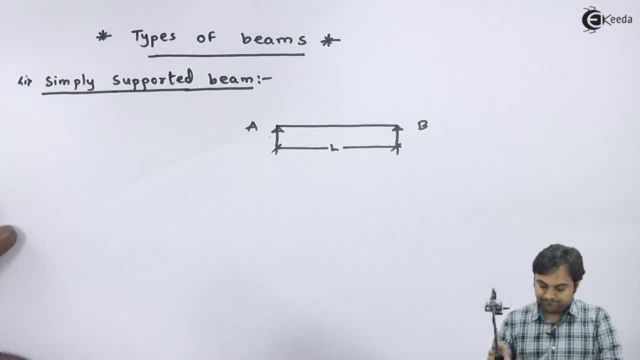 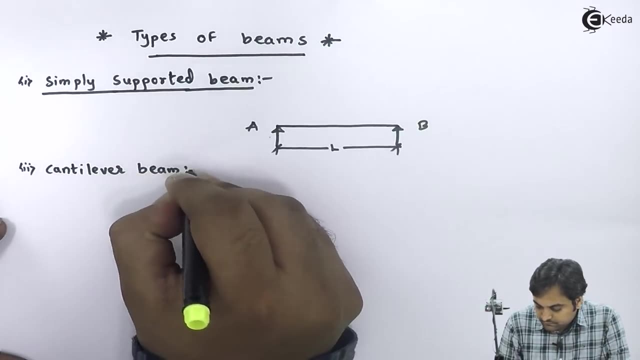 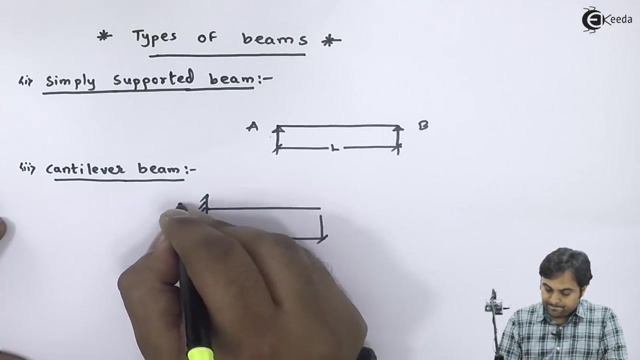 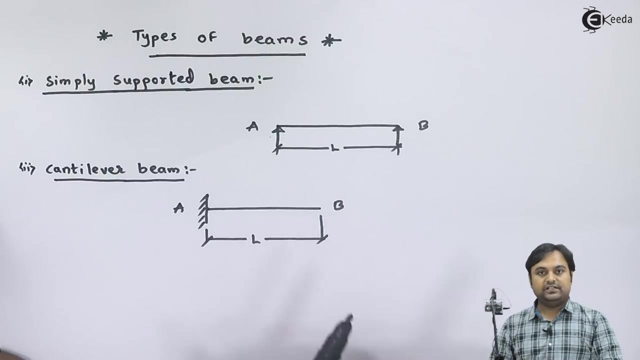 supported beam, Next cantilever beam. If we have a beam which is fixed at one end and free at the other end, that beam is called as cantilever beam, Next cantilever beam. If we have a beam which is fixed at both the ends, that kind of beam is called as fixed. 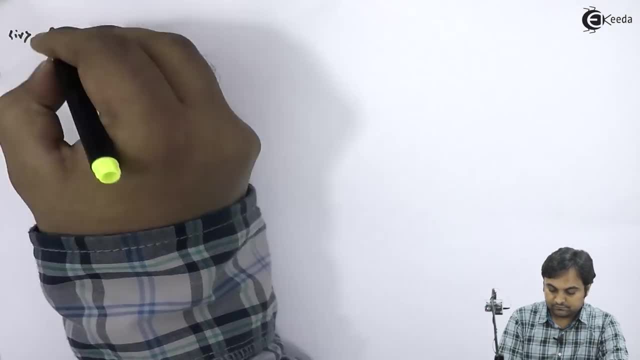 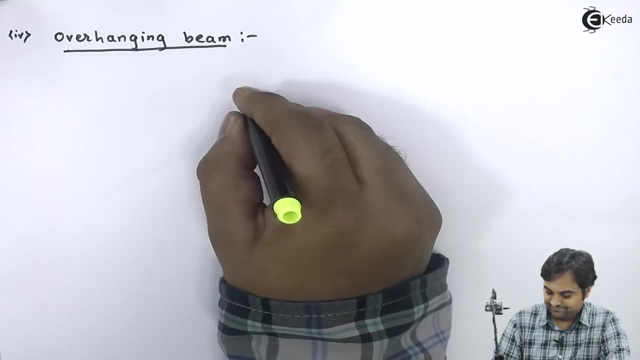 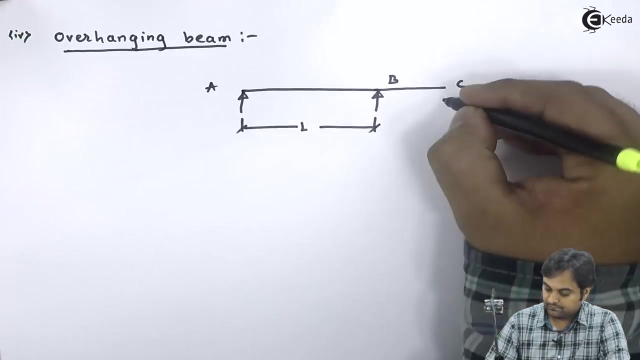 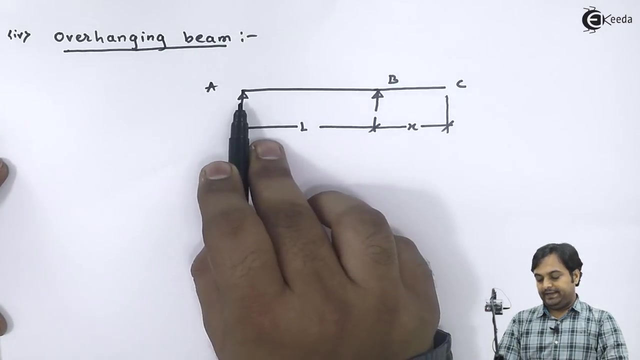 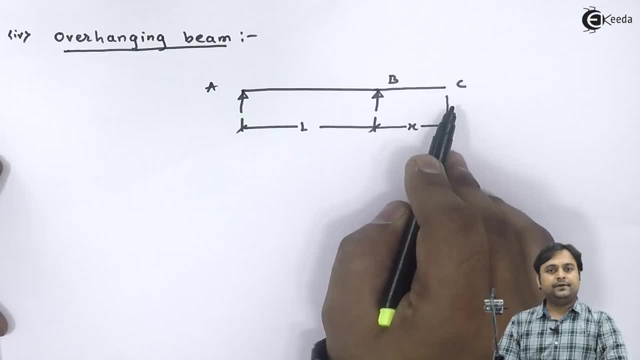 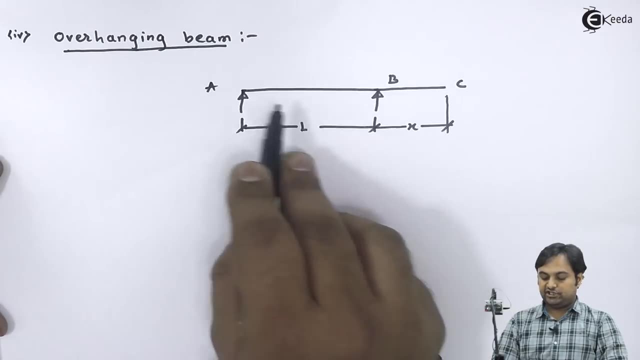 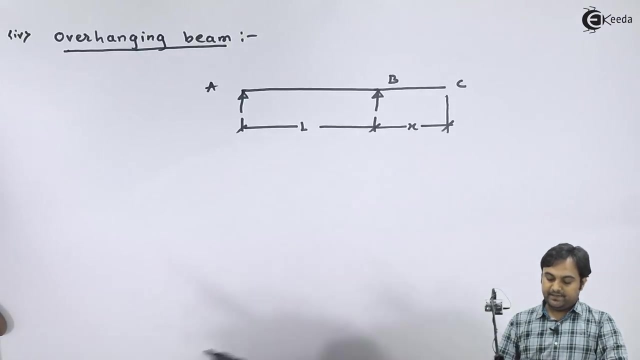 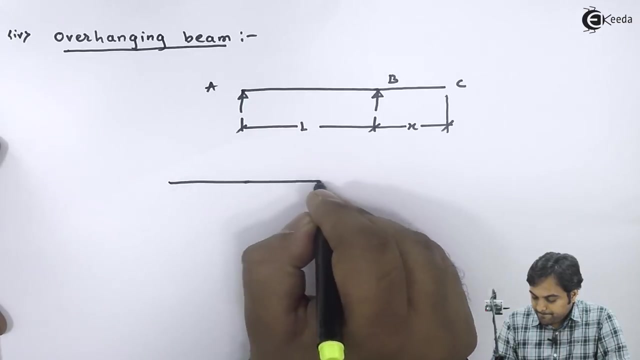 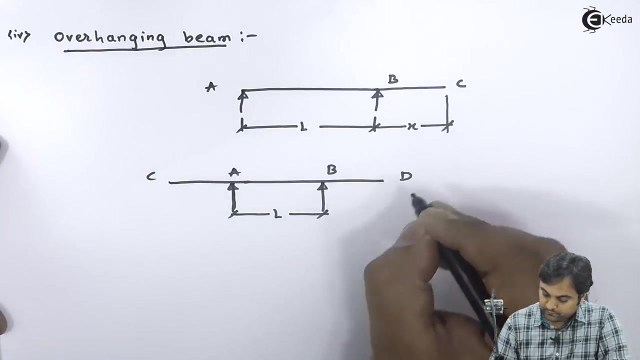 beam B. C portion of the beam is hanging. The total length of the beam is L plus X, So L portion is only supported on the side and the L of it is hanging the other way and encountered Na beam in such a way. 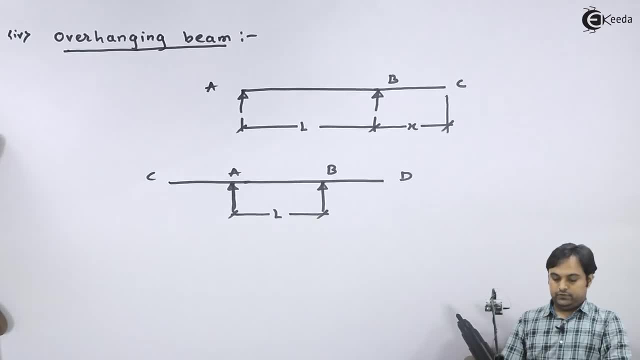 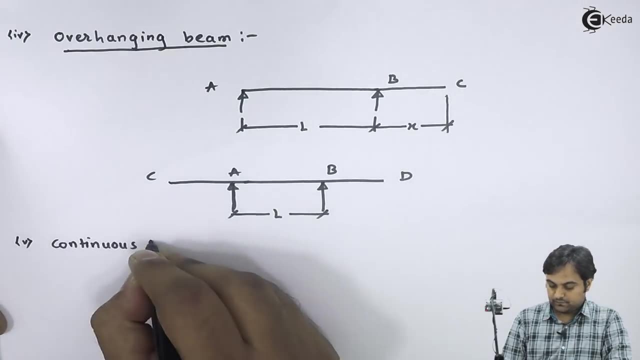 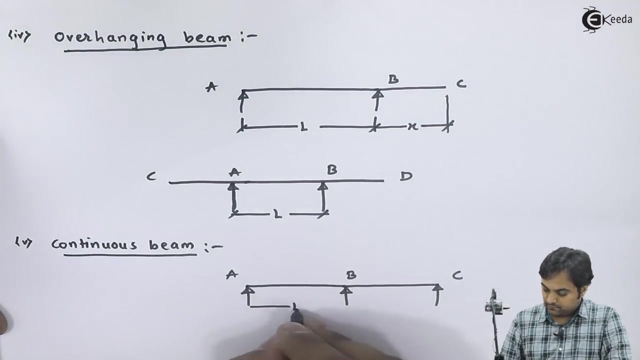 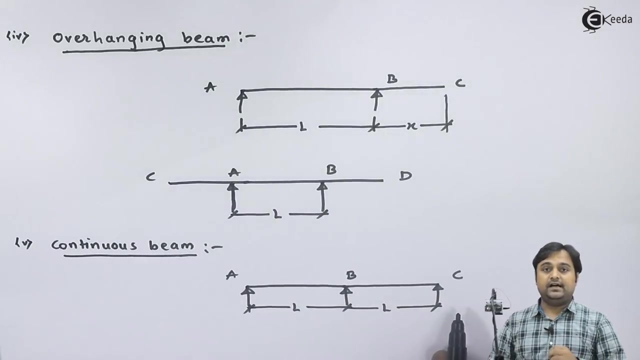 where it is overhanging from both the sides. Next we have continuous beam, a beam which has more than two supports. that kind of beam is called as continuous beam, and continuous beam is also like a simply supported beam. it is supported at the ends and, apart from 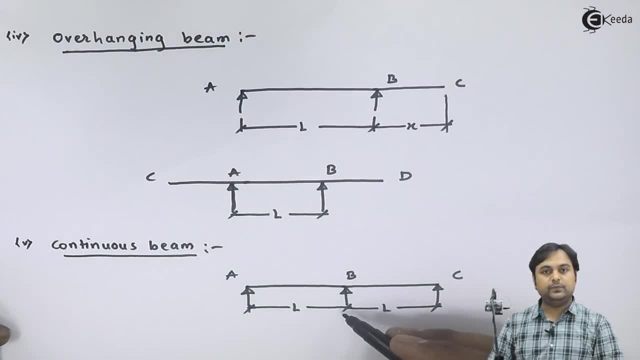 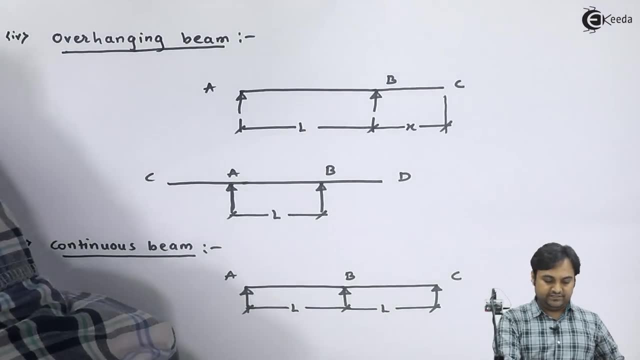 support at the ends, it should have some support in between or anywhere in between A to C. so such kind of beam is continuous beam, as we have seen in this article that here we have different types of beam. I have given you what is the example of simply supported beam. 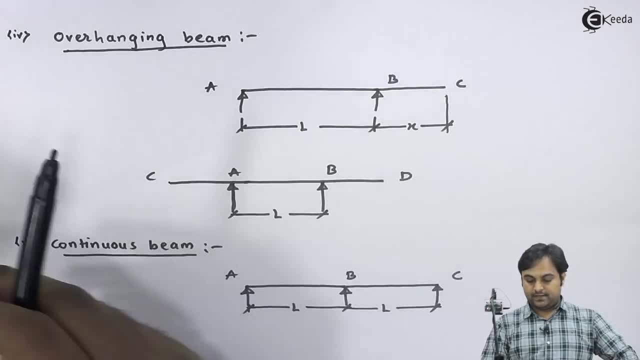 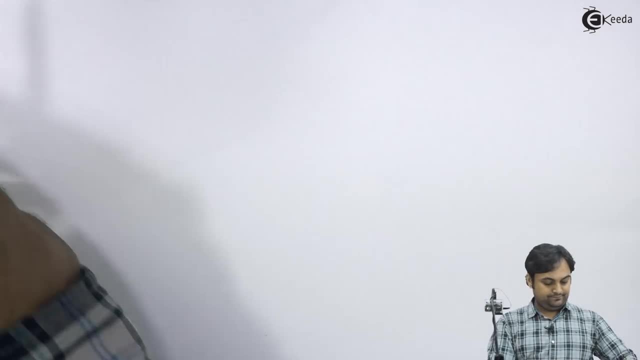 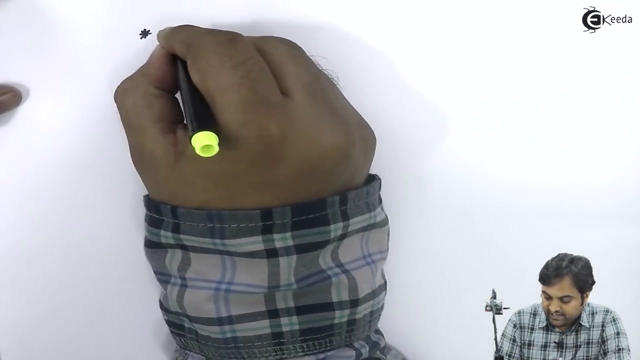 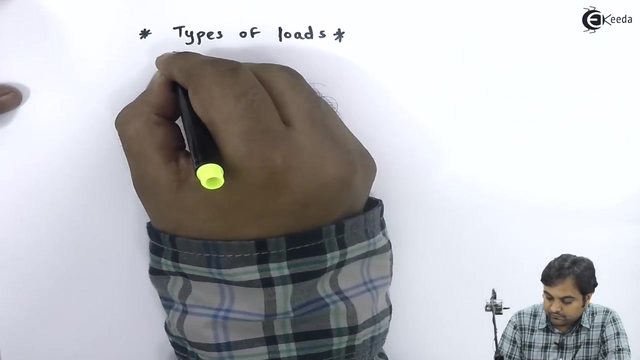 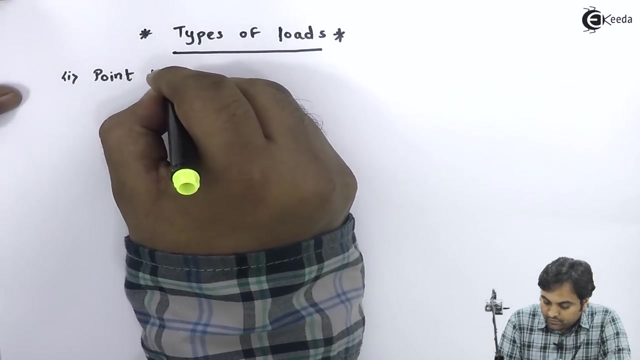 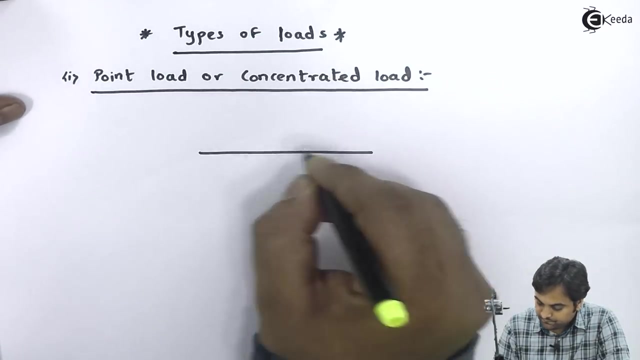 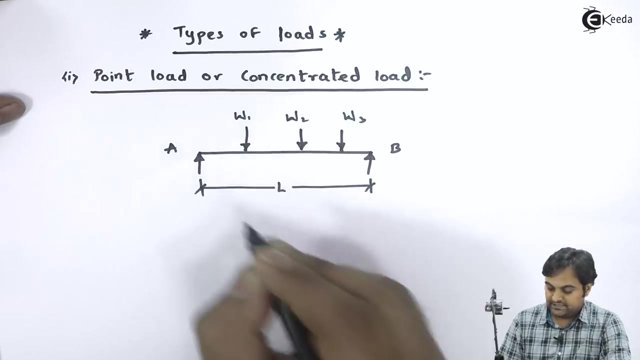 what is cantilever beam, fixed beam, overhanging beam and continuous beam. Now let me give you the types of loading similar to the types of beam. here we have types of loads. the first one is point load or concentrated load, as we see in this diagram. here we have 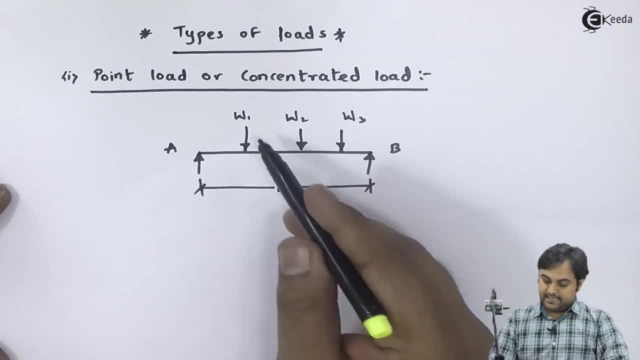 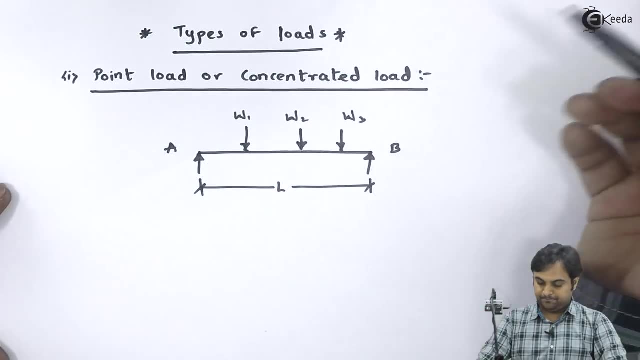 simply supported beam, supported at A and B. if the loading is in such a way that it acts at a point, like we can see, w1 is acting at a point, w2 is acting at a point, similarly w3. so here you can say that, since load is, 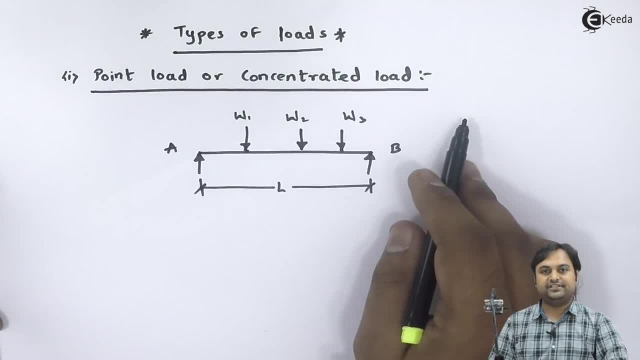 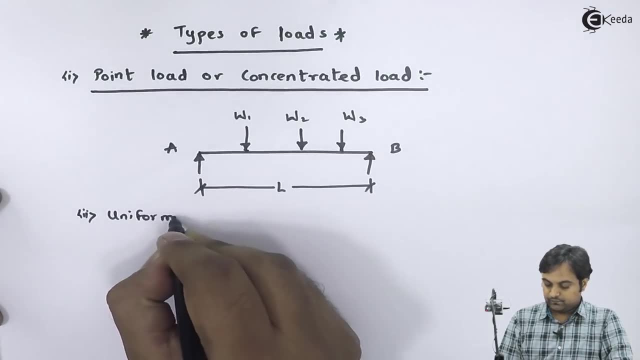 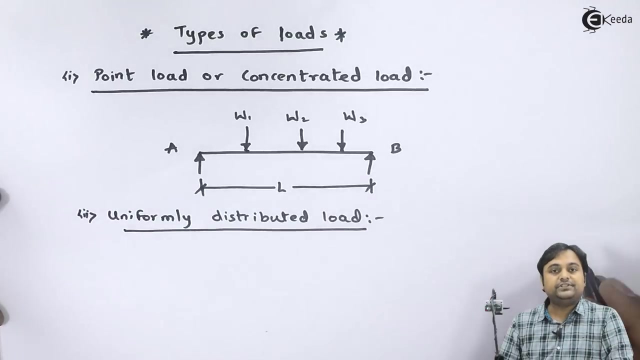 acting at a single point. it is called as point load or concentrated load. Next is uniformly distributed load: Uniformly distributed load. it has also denoted as UDL, UDL. like if I have a simply supported beam called as AB having length L, then 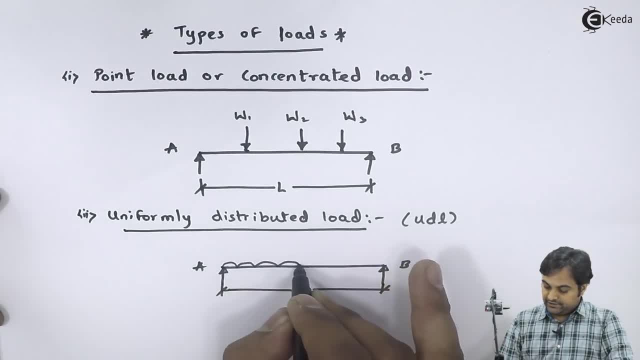 uniformly distributed load is acting throughout the length of the beam. it is not acting at one particular point like concentrated load. it is there throughout the beam and its intensity is given as W. it would be in terms of Newton per meter- and this UDL. we never use this UDL. 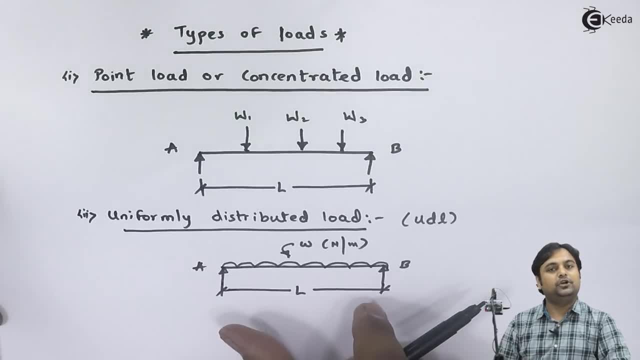 in the problem as it is, we would be converting this UDL into point load. once we are into the problems, I would be explaining it to you: how to convert UDL into point load. after uniformly distributed load, we have the last kind of load that is called as uniformly. 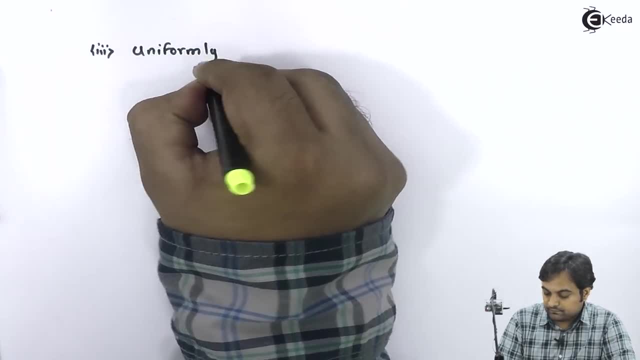 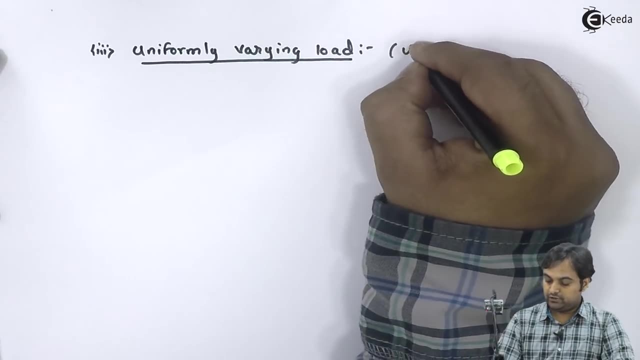 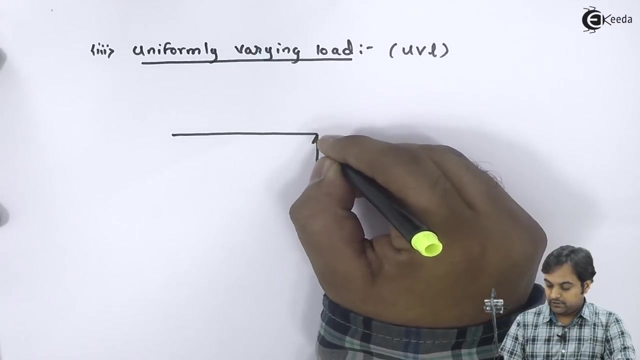 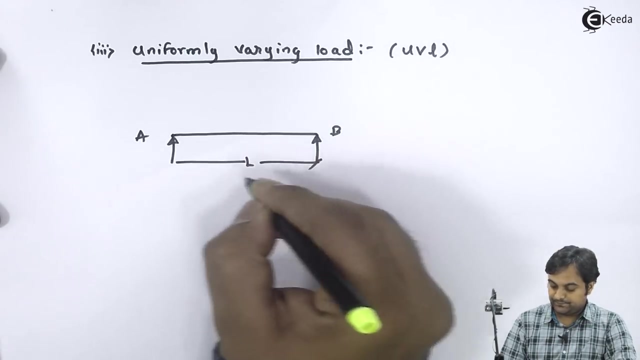 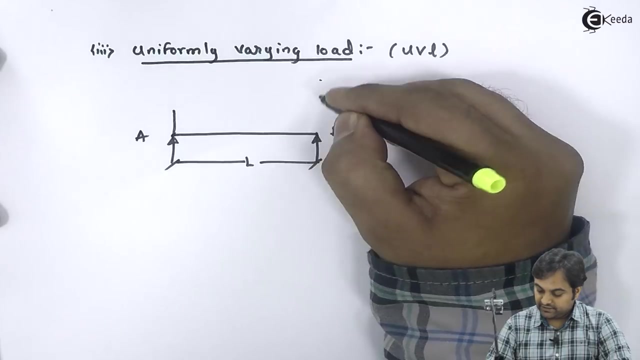 varying load. this uniformly varying load is also called as UBL. it is such a load that along the length of the beam AB, L is the length. at A, the intensity of the load is different. at B, the intensity of load is different. that is if I joined. 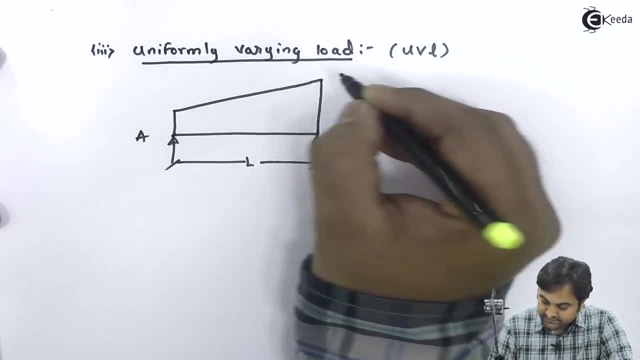 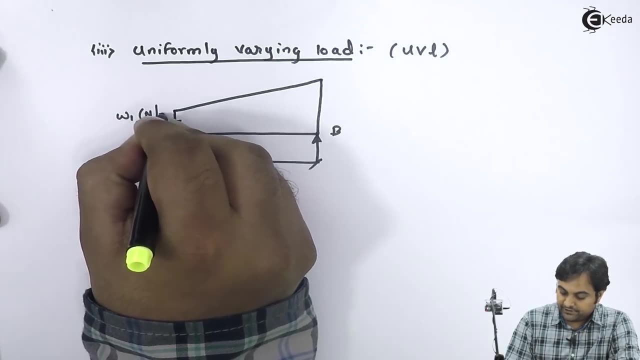 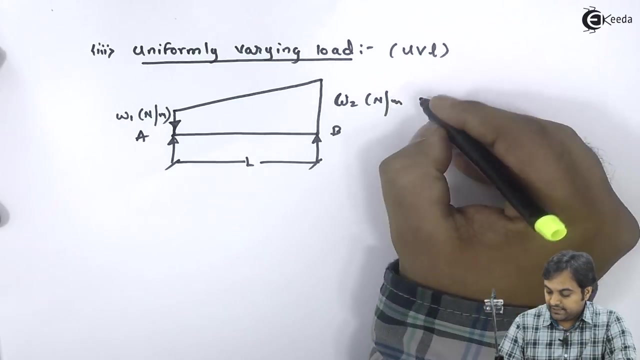 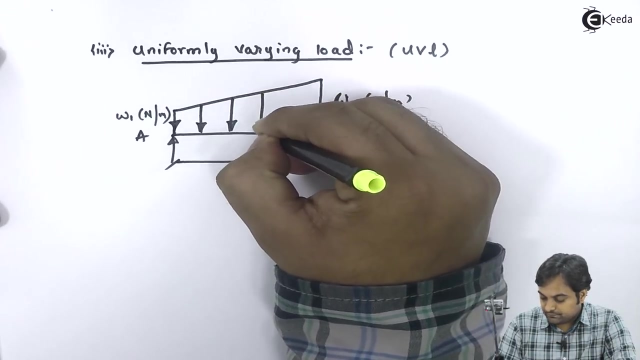 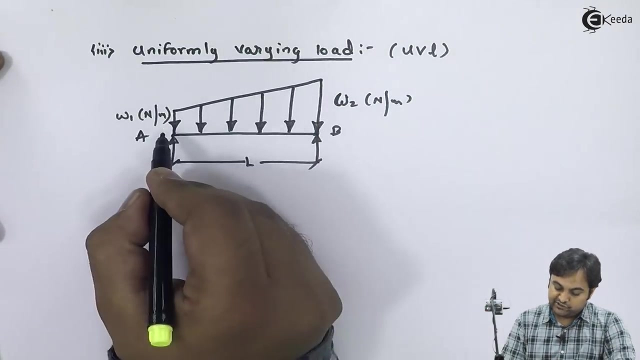 these vertical lines. I can say: at A the intensity is W1 Newton per meter, at B the intensity is W2 Newton per meter and the load is continuously increasing from W1 to W2.. So this is the uniformly varying load Suppose. here we have at W1 the load as 0, the intensity, So the 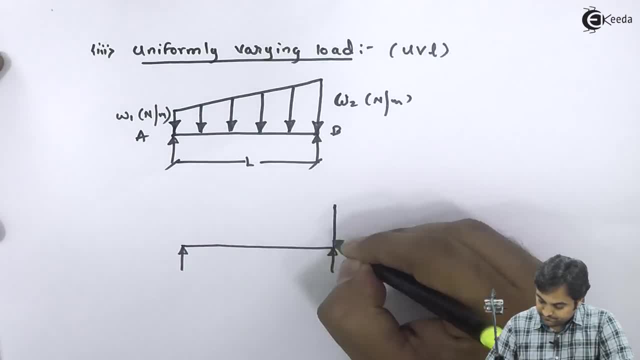 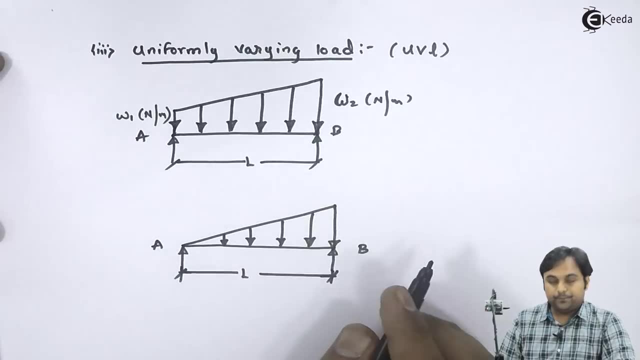 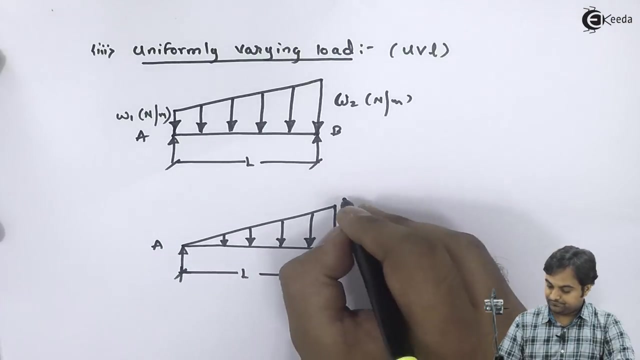 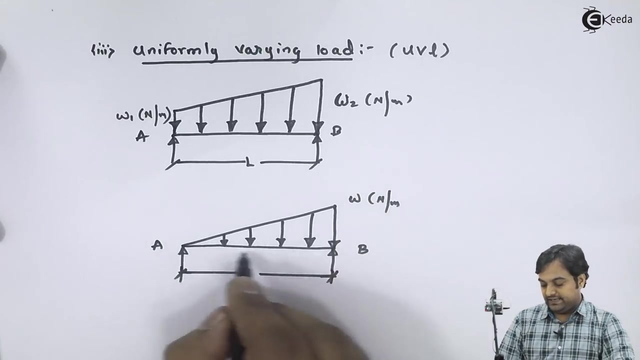 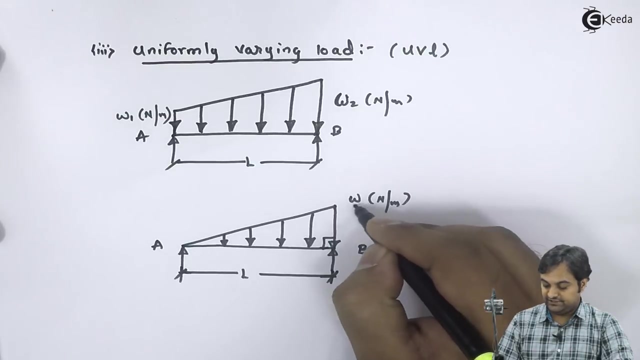 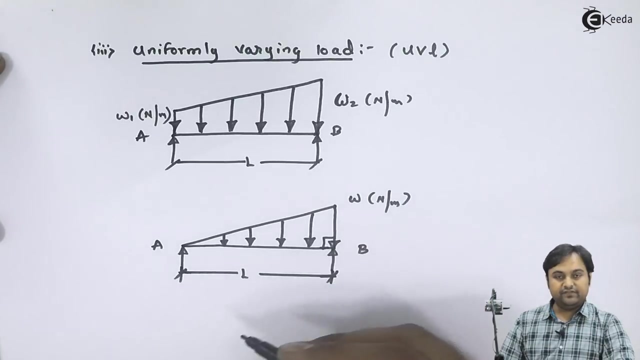 UVL will become like this. So on this kind of beam the load intensity is varying. It is W Newton per meter And it behaves like a right angle triangle where base of the triangle is considered as the intensity of load, which is W Newton per meter. L is the length, So we can even convert. 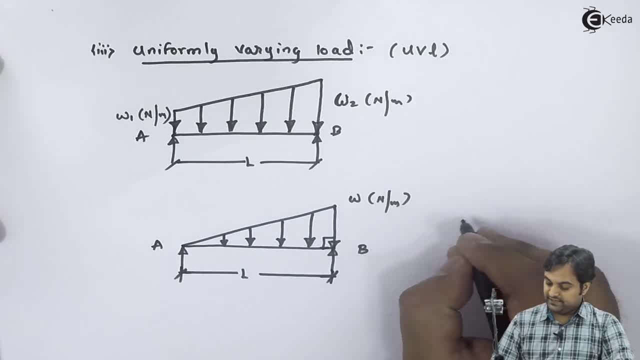 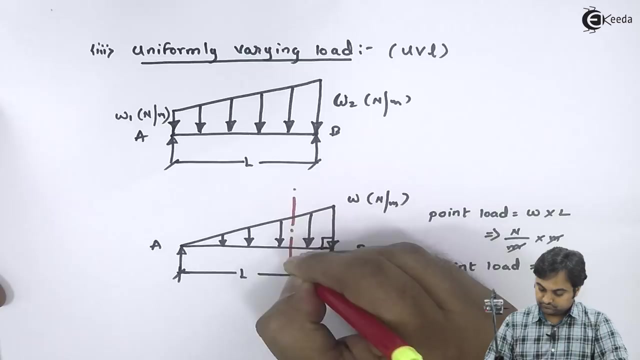 this UVL into a point load by saying that point load is equal to W multiplied by L, where W is in Newton per meter length is in terms of meter. So meter meter gets cancelled out and we have point load in terms of Newton And this point load would be acting at one-third. 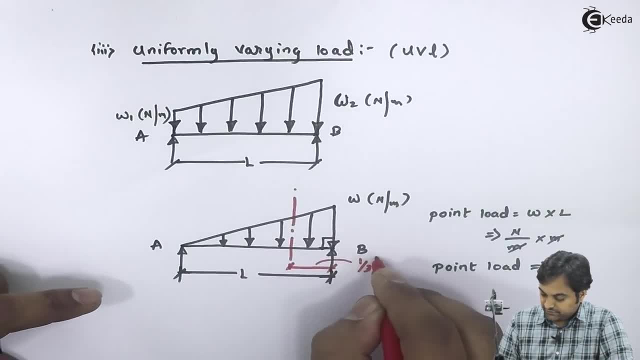 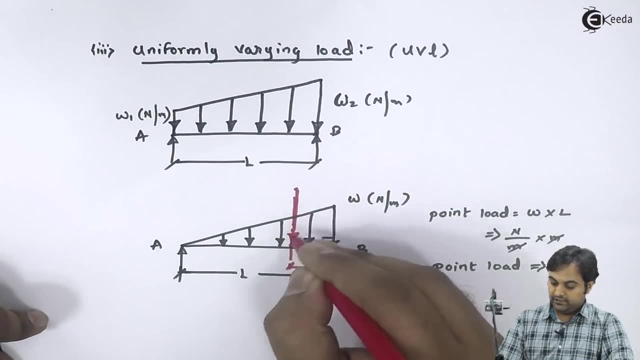 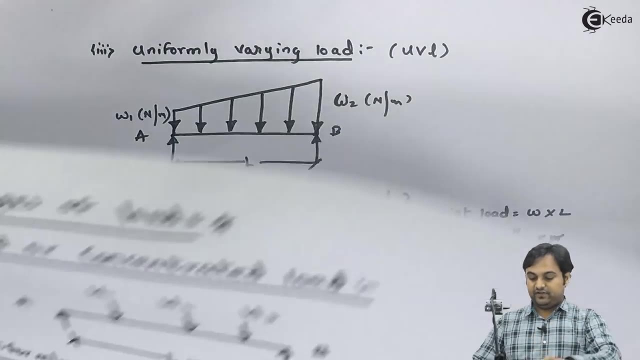 from base, That is one-third of L. So this would be the point of action of the UVL, which is converted into a point load. So with these concepts, that is, I have given you all the types of load, point load acting.